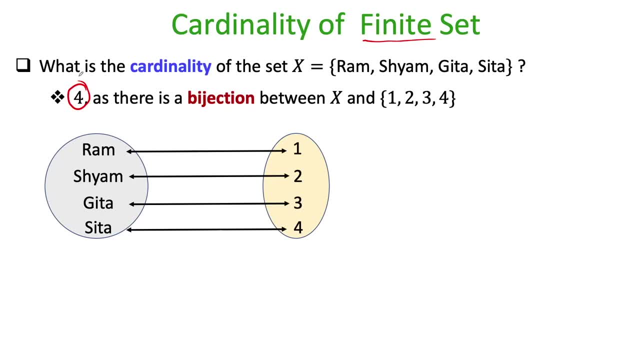 Another way to put it is as follows: We can say that the cardinality of the set X is 4, because there is a bijection between the set X and the set consisting of the elements 1,, 2,, 3,, 4.. So there can be many bijections possible between the set X and the set 1,. 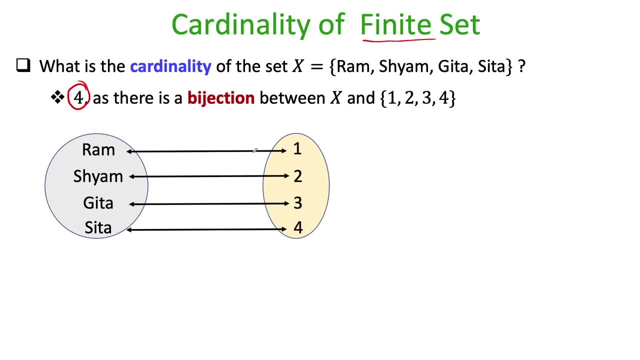 2, 3, 4.. One of the bijections could be where the element Ram is mapped to 1, Shyam is mapped to 2, Gita is mapped to 3 and Sita is mapped to 4.. You can have a bijection where Ram is mapped to 2, Shyam is mapped to 1, and so on. 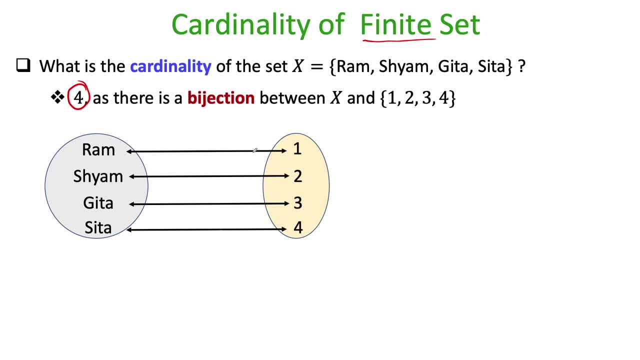 That is also a possible bijection. But since there is a bijection between Ram Shyam Gita and Sita in the set 1,, 2,, 3,, 4, we can say that the cardinality of the set X is 4, because 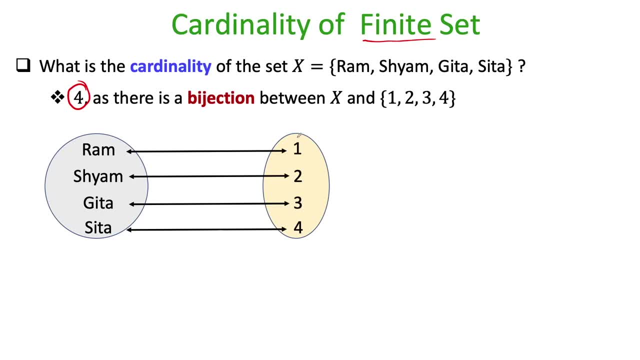 I can say that whichever element from the set X is mapped to element 1, that is the first element of set X. Whichever element from the set X is mapped to element 2, that is the second element of set X, and so on. That is why the cardinality of this set X is 4.. 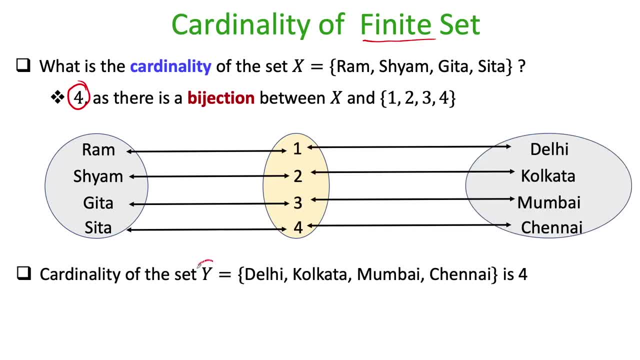 Now, due to the same reason, if I consider another set Y consisting of the elements Delhi, Kolkata, Mumbai and Chennai, its cardinality is also 4 because it has 4 elements. Or another way to put it around is that there is a bijection between the set Y and the set X, So the cardinality 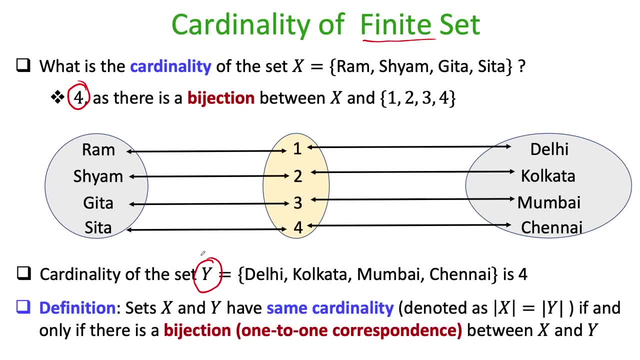 of X- if you see details in the carton lines- is like this: Based on this example, we can formulate the following definition: We can say that two sets, X and Y, have same cardinality, and for that we use this notation. Remember that this notation denotes cardinality of Y, So if the set X and sets Y have same, 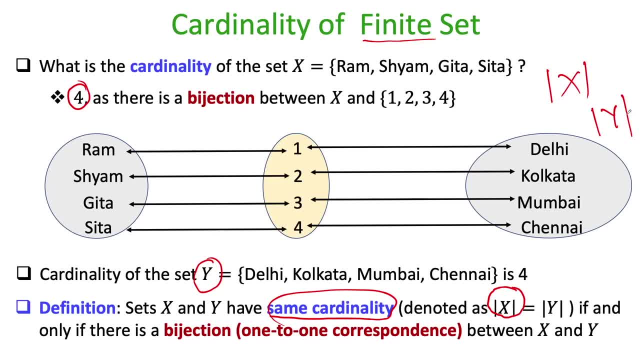 cardinality. we use this notation Now what about the other applications? These are test cases. Let us see that first. How many sets, when asked by the定ال 노 or килowatt number, that there will be different items? Let us see in that example as well: The initial也оръе Y is 10.. The total volume of 50 to 2100 volume. Now let us donate 50 to 20 people. Remember that the set S is 35,, 60 to 2 and we Composed Despite this equation, because over 5 are the words 불겠marked. 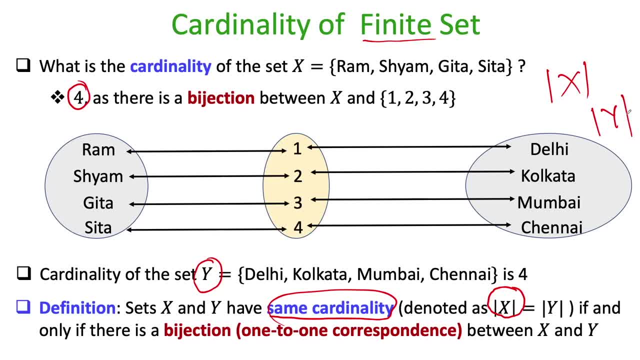 representation that their cardinality are equal. And when can we say that their cardinality are the same? We can say that provided there is a bijection or one-to-one correspondence between the set X and the set Y. So if I take this example here, the set X and the set Y have the 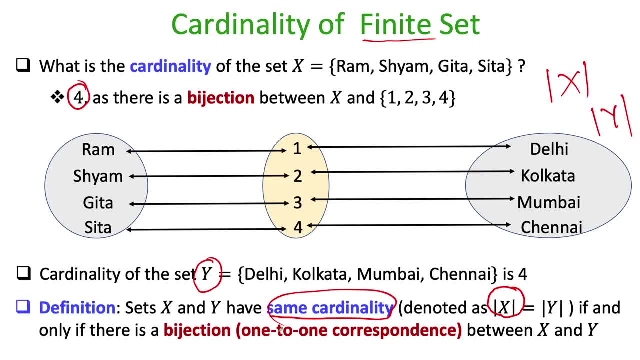 same cardinality because they have the same number of elements, namely 4.. But if I see it in terms of a function, then I can say that the set X and the set Y have the same cardinality because there is a bijection between the set X and the set Y. 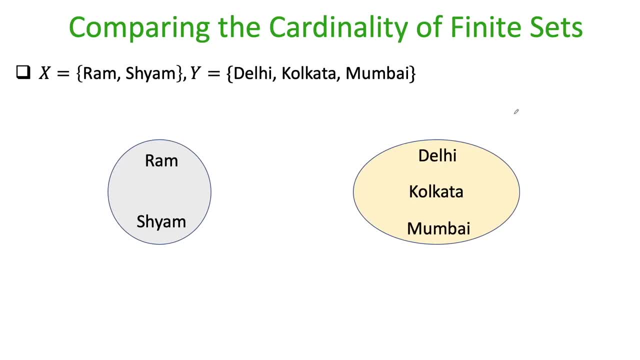 Now, how do we compare the cardinality of finite sets? So if I am given the set X and the set Y, it is easy to see that the set X, its cardinality, is less than the cardinality of set Y, Namely, 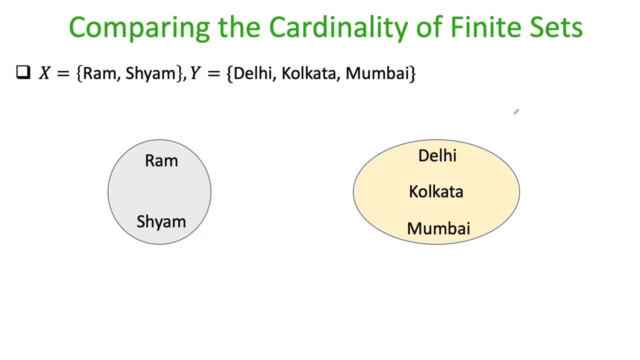 the number of elements in the set X is less than the number of elements in the set Y. That is why the cardinality of the set Y is less than the cardinality of the set Y. The cardinality of X is less than the cardinality of Y, But if I view the same thing in terms of a, 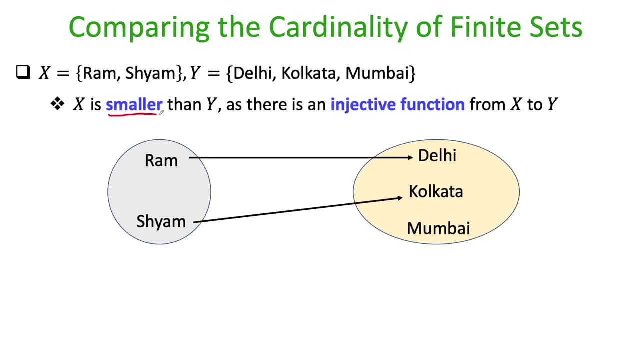 function. I can say that the set X is smaller than the set Y in terms of size because there is an injective function from the set X to the set Y, So there can be many injective functions. One possible injective mapping I can define as Ram getting mapped to Delhi and Shyam getting 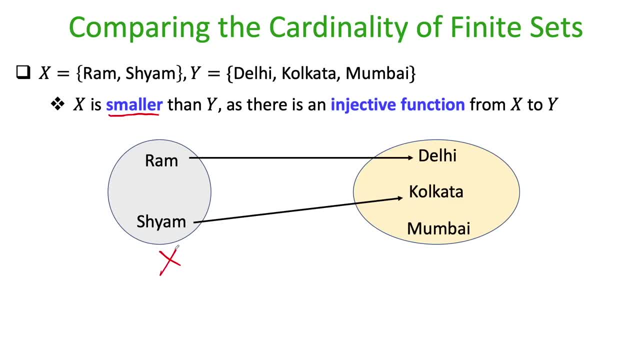 mapped to Kolkata. That means you take any element from the set X, it will have a image, a distinct image from the set X. So that is the cardinality of X And distinct elements from the set X will have distinct images. So that automatically ensures 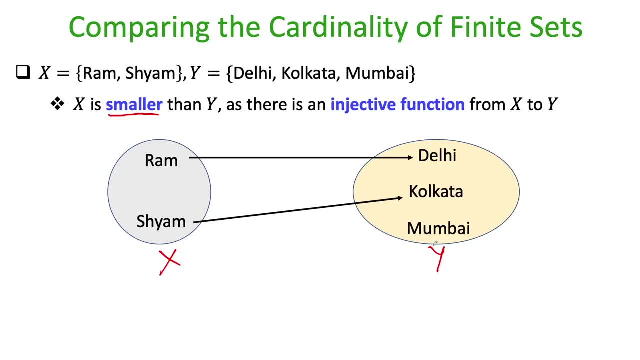 that the number of elements in the set Y has to be at least as large as the number of elements in the set X. So, based on this example, I can give the following definition. I can say that the cardinality of the set A is less than or the same as the cardinality of set B. 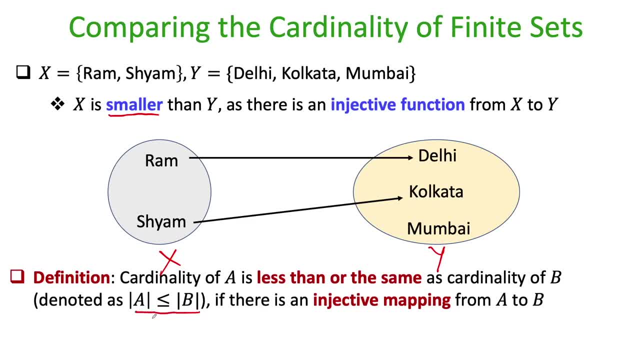 And we use this notation, the cardinality of A less than equal to cardinality of B, Provided there is an injective mapping from the set A to B. You might be wondering why I am using less than equal to notation here, because there might be more elements in the set B compared to. 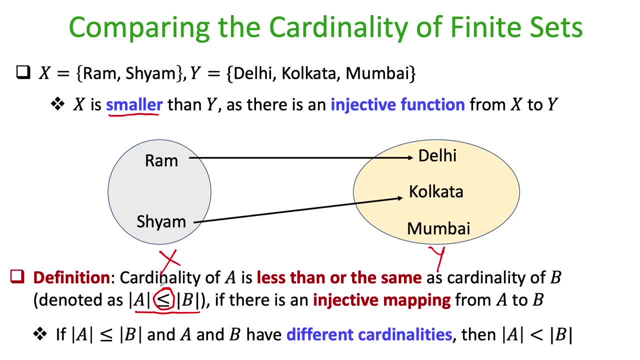 the set A. That is why they are less than equal to notation. Now, if the set A cardinality is less than equal to cardinality of set B and the cardinality of the set A and the cardinality of set B are different, then clearly it implies that the cardinality of the set B is less than or equal to. 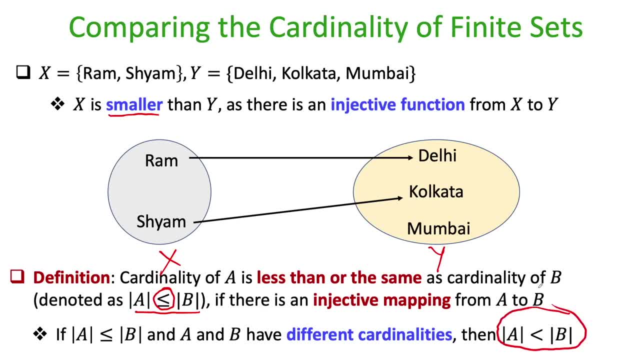 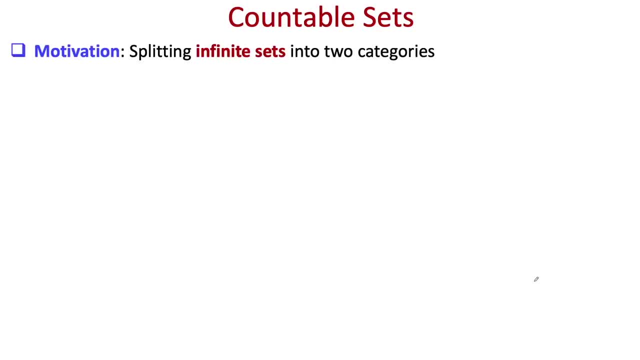 the cardinality of the set A. So now, what are countable sets? So before going into the definition of countable sets, let us see some motivation why we want to study countable set. The whole motivation behind countable sets is that we want to split the study of infinite sets into. 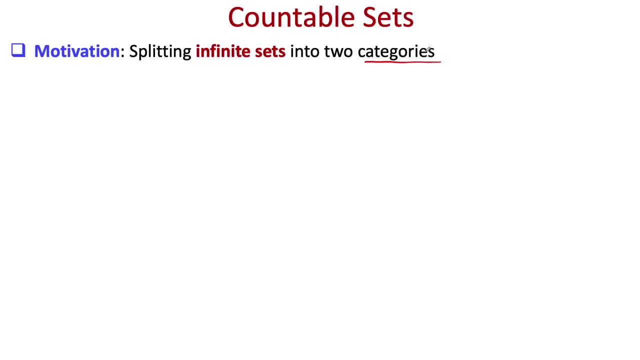 two categories. What are infinite sets? On a very high level, they are sets which has infinite sets. So we want to split the study of infinite sets into two categories. So what we want to do is we want to categorize this infinite sets into two categories: Sets which 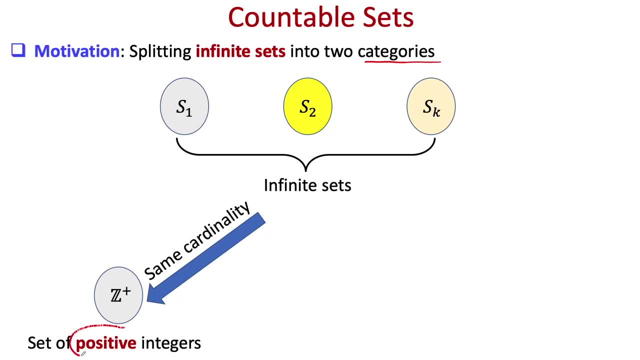 have the same cardinality as the set of positive integers, and a set of positive integers are denoted by this notation, zp. So we want to categorize this infinite sets into two categories. So what we want to do is we want to divide zp by zp plus and we want to categorize the infinite sets into other. 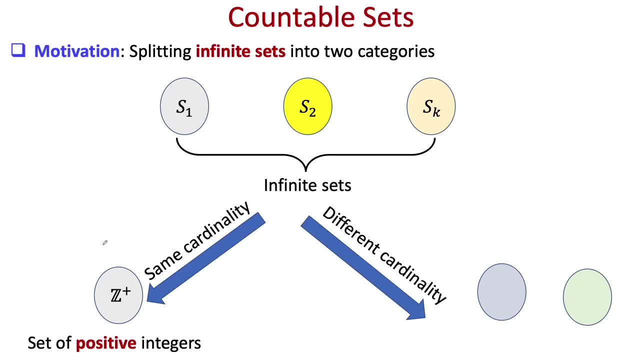 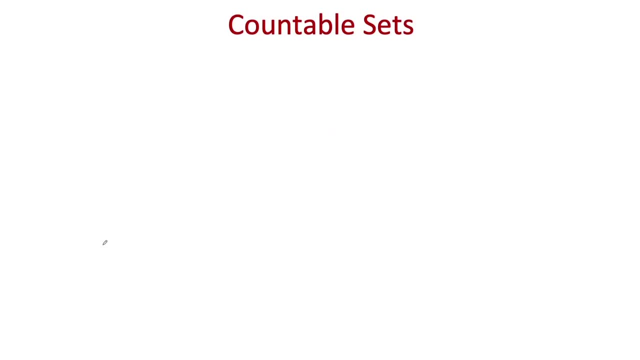 category which have different cardinality than the cardinality of the set of positive integers. That is the whole motivation of defining this notion of countable sets. So when exactly we say a set A is countable? We say a set A is countable. 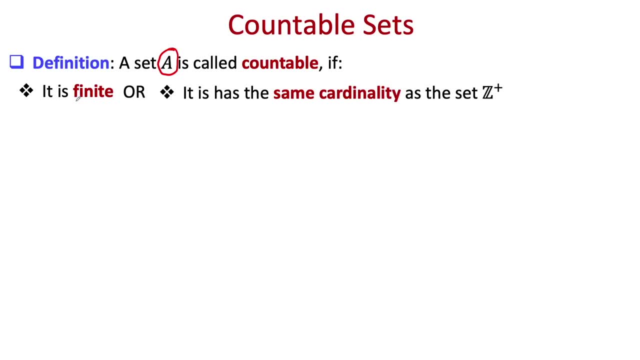 it satisfies one of the following two conditions: Either it has to be finite, namely it has finite number of elements, or it has the same cardinality as the set of non-negative integers, namely the set of positive integers. to be more precise, It has to be the same cardinality as the set 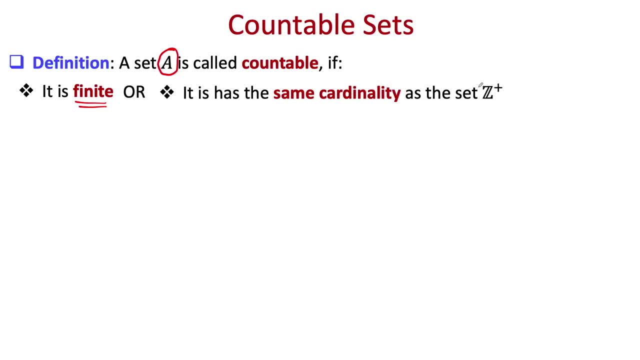 of positive integers. If one of these two conditions are satisfied, then we say that the set A is countable, Whereas if a set A satisfies neither of the above conditions, then we will say that the set is not countable. So if you are given an infinite set, say S. 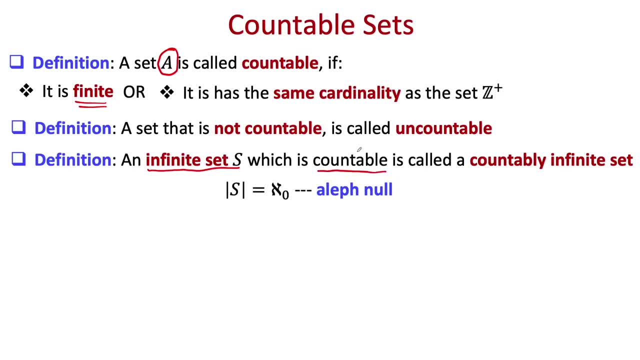 which is countable. So since the set is infinite, that means definitely we cannot say how many elements the set S has. But if it is cardinality is same as the set of positive integers, then we will call the set A as countable. So if you are given an infinite set, say S. 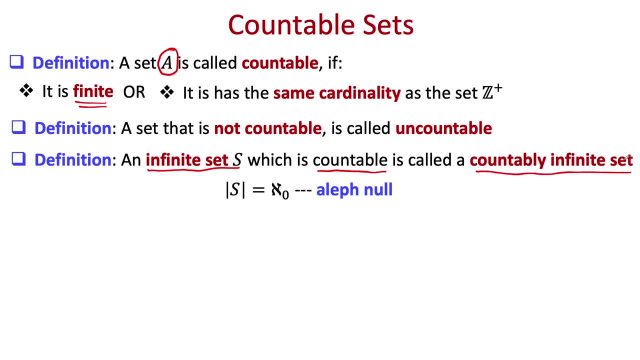 to be countably infinite. So we have countably finite sets and we have countably infinite sets. So countable sets can be categorized into two categories. Either they can be countably finite- that means its cardinality is finite- or there are infinite. 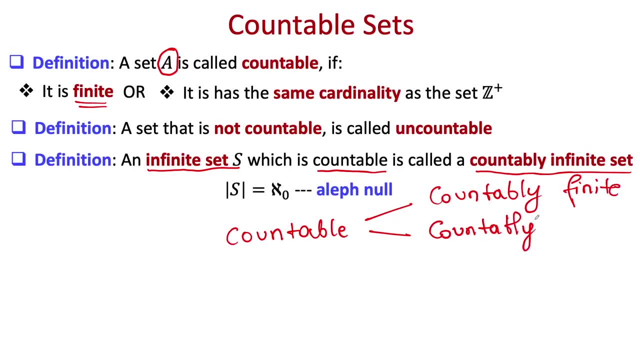 number of elements in the set, But they are countably infinite. So if you are given an infinite set, say S is countable in the sense that their cardinality is same as the cardinality of set of positive integers, Whereas if the set is not countable, then we will call it. 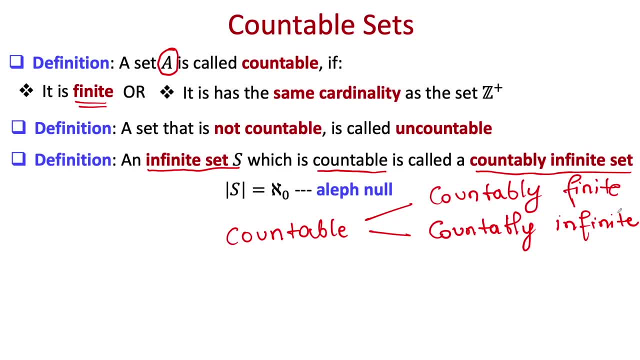 uncountable. So if we are considering the second category of countable sets, namely infinite sets whose cardinality is same as the set of positive integers, then we use this notation, aleph null, to denote the cardinality of such sets. So this is an Hebrew character, this aleph character and 0 denotes the null feature here, So the 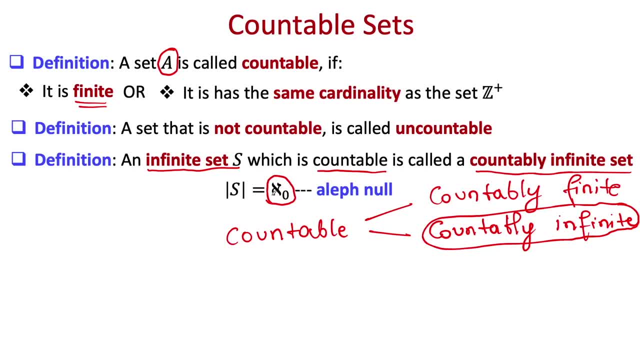 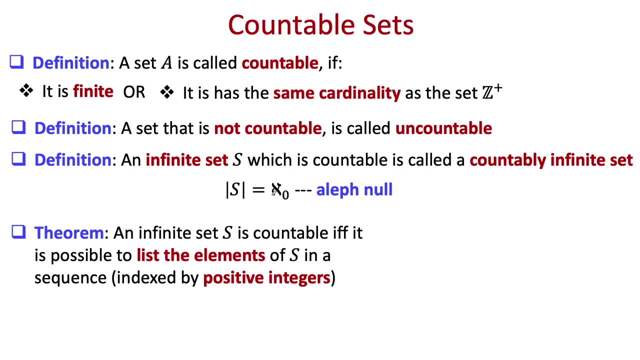 cardinality or the size of the set of positive integers is called as aleph null, and if your set is countably infinite, then its cardinality will be aleph null. So now we can quickly prove this theorem, which will be very useful later on. if you are given a set, S, which is 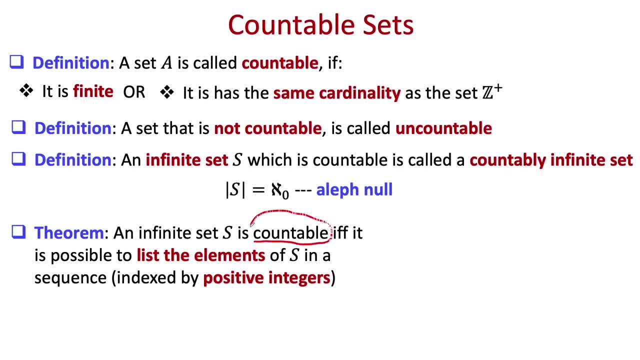 countable. So if the set S is countably infinite, then it is countable if, and only if, it is possible to list the elements of the set S in a sequence indexed by positive integers. So what it basically says is that even if you have infinite number of elements in the set S, it is countable. 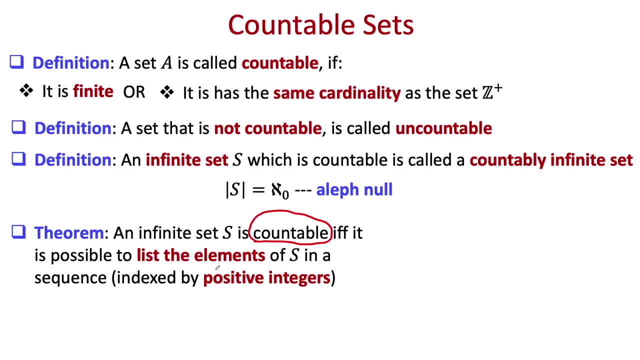 in the sense I can give you a sequencing, I can give you a method, a well defined method, according to which you can list down the elements of the set S, And the method is well defined in the sense that no element of the set S will be missing. 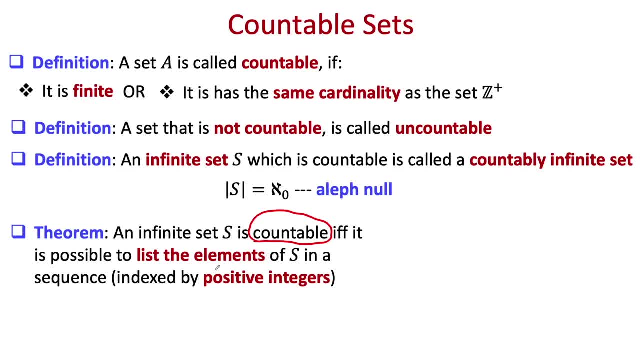 as per the definition of that sequencing. that means the way I will give the definition of the sequencing or the listing of the element. each element of the set S will appear somewhere in that sequence. In that way it is a well defined sequence and no element will be repeated. 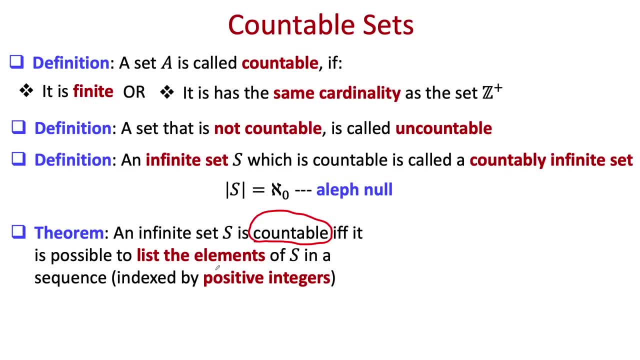 in that sequence. So let us put: and in that sense only my set is countable, even though it has an infinite number of elements. So the proof of the theorem is very simple. since your set S is countably infinite, that means its cardinality is same as the set of positive integers and the set of positive 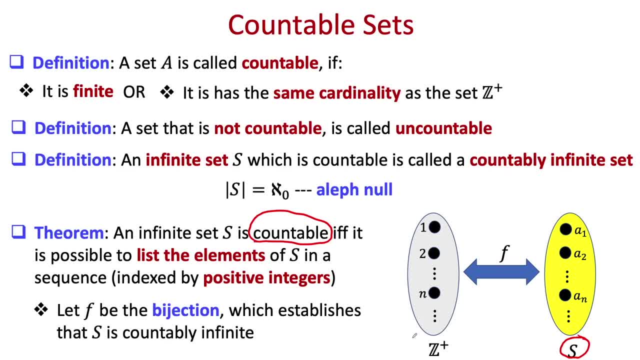 integers are 1,, 2 and up to infinity and there has to be a bijection. call that bijection as little f between the set of positive integers and your given set S. Now if in that bijection the element a 1 is mapped to integer 1 and element a 2 is, 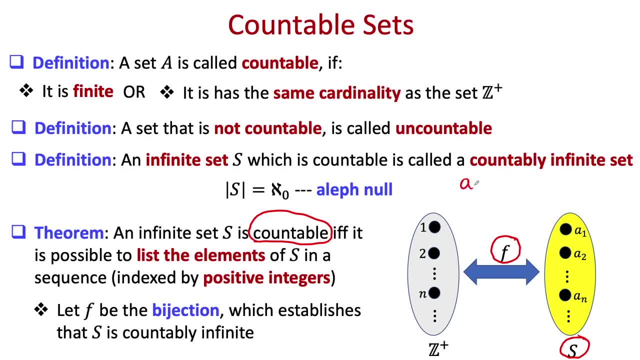 mapped to the integer 2 and so on, then what I can say is that a, 1, a, 2, a, i a n is a valid sequencing or valid listing of the elements of the set S. Why it is valid? because, first of all, no element in this sequence. 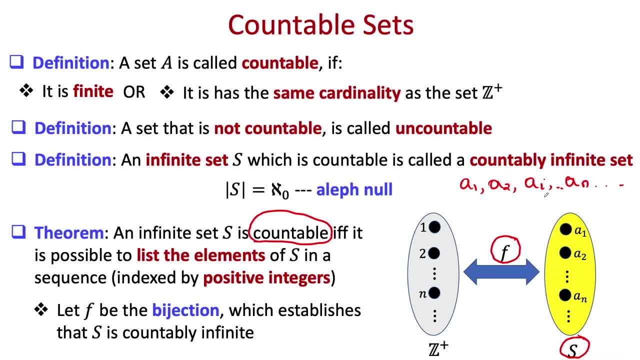 Is repeated, and if you take any element in the set S, it will appear somewhere in this sequence. It's not the case that no element will be missed in this sequence. Okay, even though they are an infinite number. Okay. So what this theorem basically says is that if you want to show a 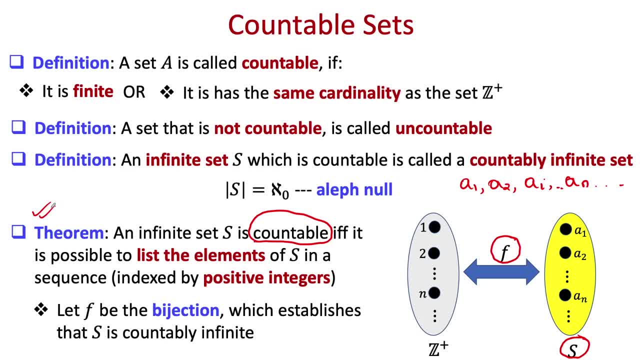 Given set to be countable, and there are two ways to do that. If it is finite, just find out the cardinality of that set. But if it is infinite, then the only way you can show it is countable is either show a bijection Or you give me a very defined sequence, a very defined way of sequencing the elements of that set. 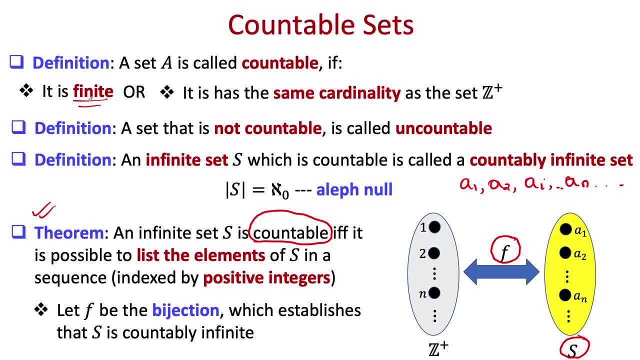 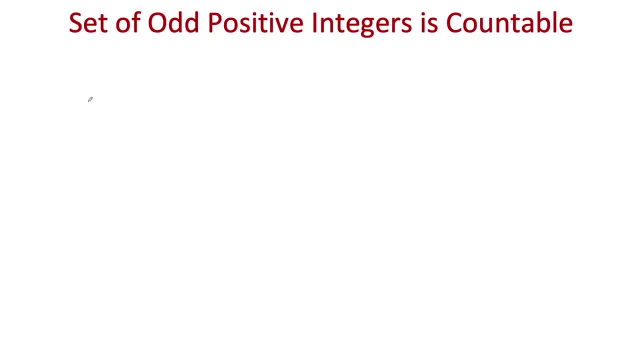 Okay, that is equivalent to saying that you are giving me a bijection between the set of positive integers and the given set. So now, based on this definitions, let's see some examples of countably infinite sets. so I start with the set of odd positive integers and 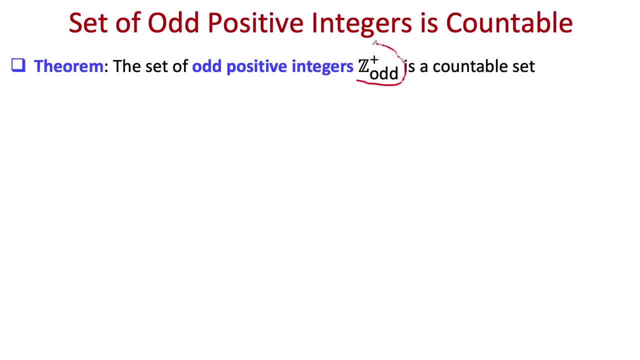 Let me denote the set of odd positive integers by this notation and my claim is that the set of odd positive Integers is a countable set. so Might look, the statement might look- very non-intuitive because definitely you have more integers than the set of Odd positive integers. right, the set of integers. if I consider the set of positive integers, 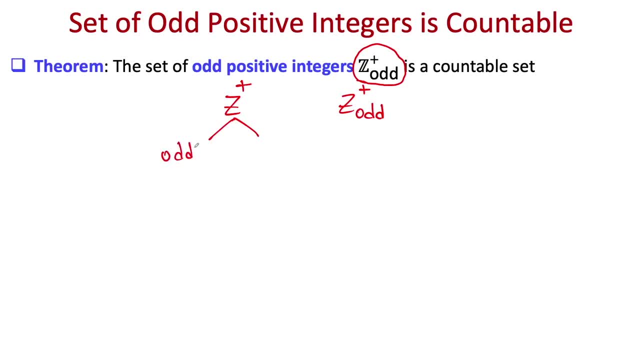 To be more precise, then it has both odd integers as Well as even integers- okay, and Both this sets: the set of odd positive integers and the set of even positive integers. each of them is an infinite set. What I am going to show here is that 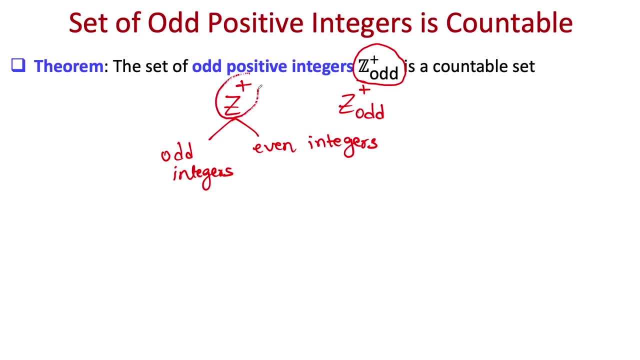 cardinality wise: the set of odd, a set of positive integers and the set of odd positive integers, their cardinalities are By showing a bijection. okay, So my bijection is as follows. so Consider the sequence 1, 3, 5, 7, Where, and like that, where the nth term in the sequence is 2, n minus 1, and so on. 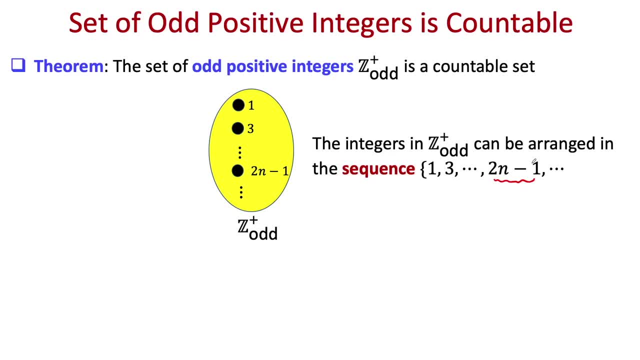 So clearly. this sequence is a sequence of infinite positive integers and each number in this sequence is odd. My claim is that this is a valid sequence For the set of odd positive integers. It's valid in the sense no element in this sequence is repeated and You take any integer from this set of positive integers, It will appear somewhere in this list. 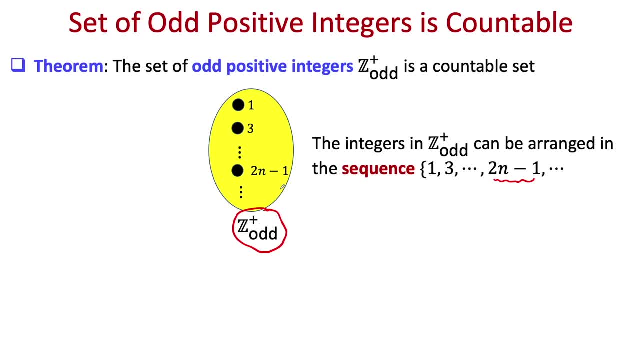 It will not be the case that you keep on Traversing this sequence infinitely, but still you never come to that element which you are considering right. It give me any element X Belonging to the set of odd positive integer. It will appear somewhere in this sequence. 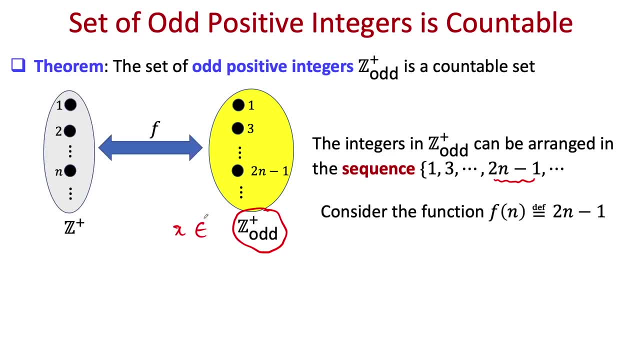 To be more precise, if you want to see the exact bijection between the set of odd positive integers and a set of Positive integers, you consider the mapping f of n, where f of n is 2n minus 1, And it is very easy to see that the function is injective. 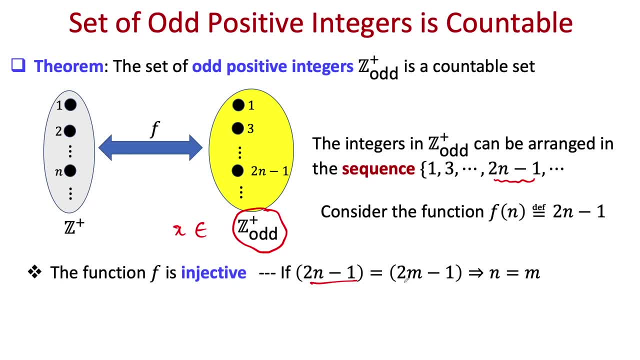 Because if you take the integers 2n minus 1 and 2n minus 1, and if they are same, Then that's possible only if your n is equal to n and clearly the function is subjective as well How you take any element y. 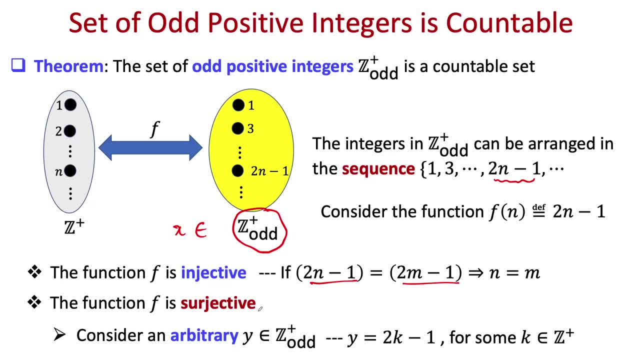 Belonging to the set of odd positive integers corresponding to that element y. you have, That element y can be written, since it's it's an odd positive integer. It can be written in the form of some 2 times k minus 1 for some k in the set of positive integers. 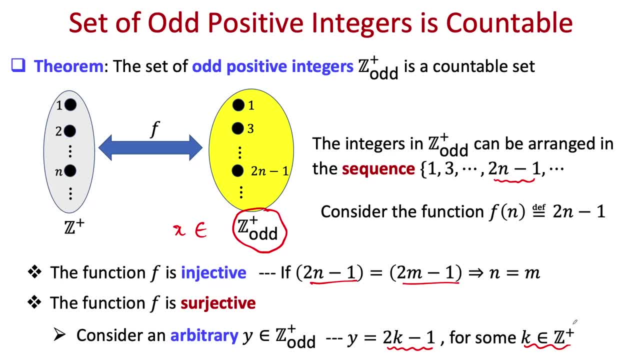 so the pre image of y will be the element k. so that's a bijection and that shows that cardinality wise, the set of odd positive integers Same as the set of positive integers, Even though intuitively you have more elements in the set of positive integers than the set of odd positive integers. 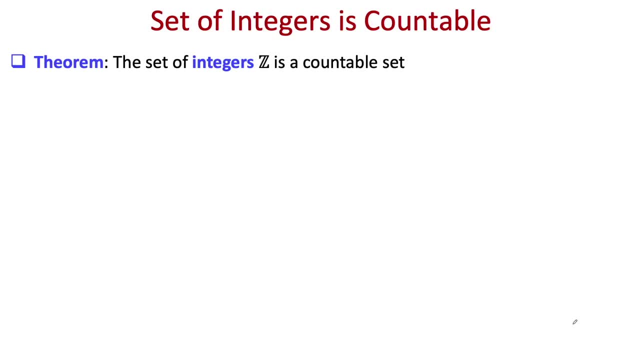 Now, what we are going to show next is Very interesting fact. we are going to show here That the set of integers is a countable set. Mind it, the set of integers has both positive integers as well as negative integers. But what we are now going to show is that, cardinality wise, the set of integers is same as the set of. 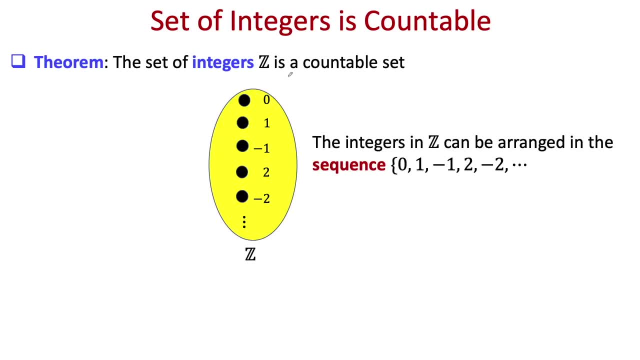 Odd positive integers. They have the same number of elements. Okay, so again, I will do it by giving you a valid sequence and also by giving you an explicit bijection. So let me first show you a sequence here. My sequence here is the following: I start with 0 and then I 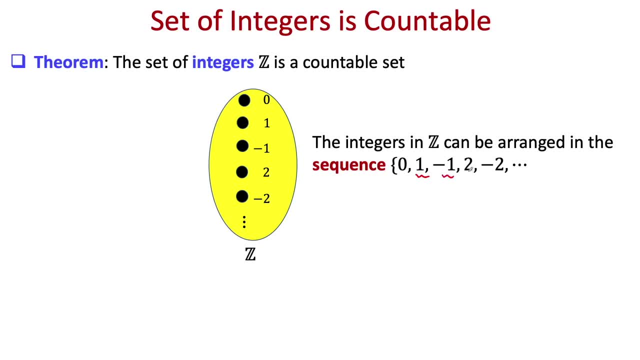 alternately List on positive numbers, negative numbers, positive numbers, negative numbers, and then I gradually go along the number line, Both in the positive direction as well as in the negative direction. My claim is that this is a valid sequence in the sense you take any integer, Okay, either it will be positive or it will be negative, and it will appear somewhere in the way I am. 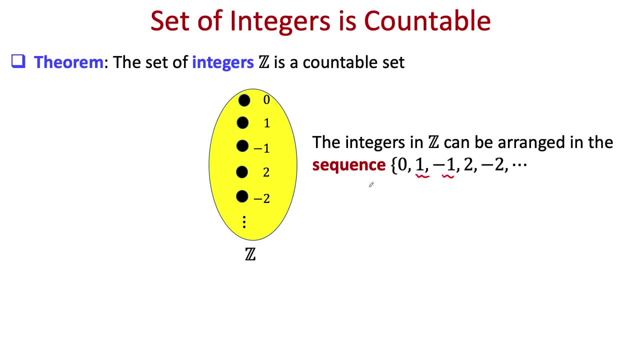 Listing down the elements here. Let me ask you a question here. You can think in your mind: If I consider a sequence where I first try to write down all the positive integers and Then followed by the negative integers, Okay, Can I consider this to be a valid sequence for listing down the set of integers? 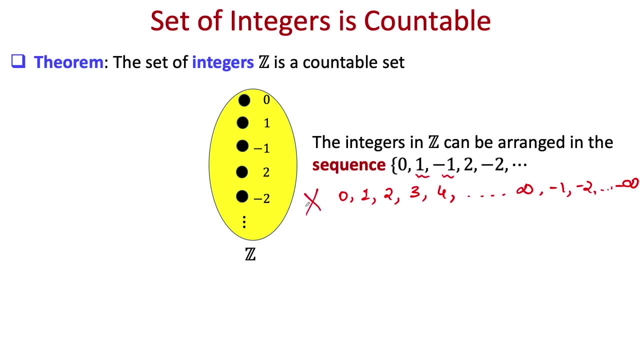 The answer is no. this is not a valid sequence. Why this is not a valid sequence? because if you take a negative number, say minus 1, You don't know where exactly minus 1 is going to appear in this list, because you are starting with the set of positive integers. 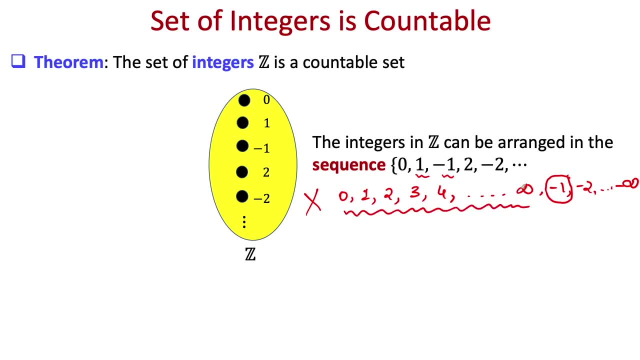 And when you are actually traversing the set of positive integers, you are going to an infinite limit. There is no Guarantee that you will come back and then start enumerating your negative integers. Okay, that in that sense this Enumeration is an invalid enumeration or invalid listing. 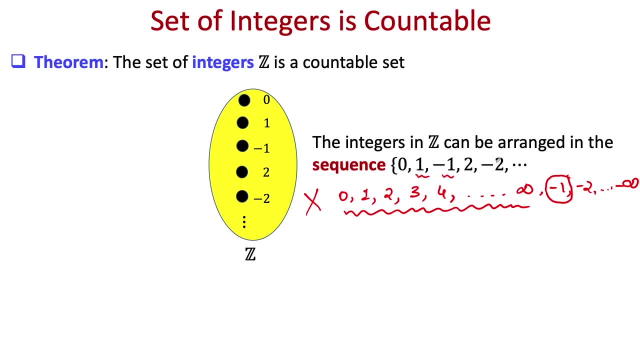 Whereas the way I have listed down the elements where I have alternatively, Alternately, listing down the positive, negative, positive, negative integers, That means along the number line: I started with 0 and then, In each step, I am listing down the next positive number and then the next negative number, then the next positive number than the next. 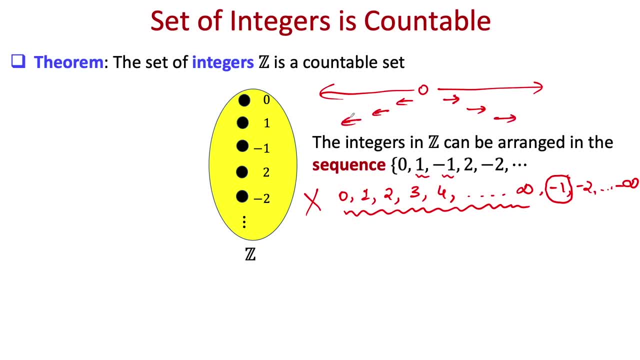 Negative number, then the next positive number than the next negative number. If I consider this sequence, then even though your Given integer, which you want to find out where exactly it is appearing in the sequence, is Very, very large, It might be appearing somewhere Arbitrary and you don't know where exactly it is appearing. It will eventually be enumerated in the sequence. You will never miss it. 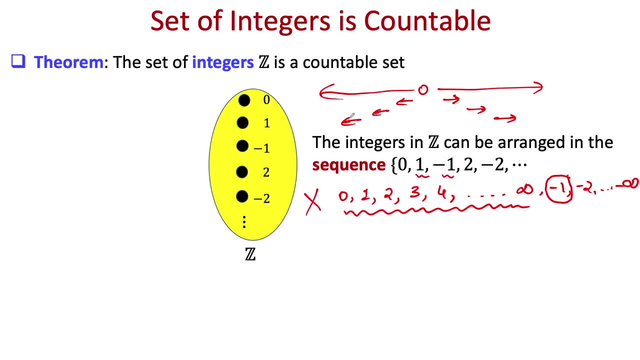 That's why it's a valid sequence in it, a valid listing, Whereas the listing that I have considered here, where I am first trying to enumerate all the positive integers, followed by all the negative integers, It's not a valid sequence. okay, Now, if you want to see an explicit bijection between the set of integers and a set of positive integers, consider the following mapping: 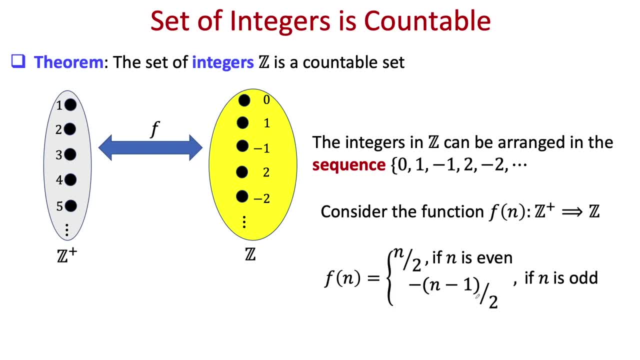 My f of n will be n over 2, provided n is even, whereas if n is odd, that means n minus 1 is divisible by 2. then my mapping will be minus of n minus 1, and It is a straightforward exercise for you to verify that indeed, this mapping f is a bijection. 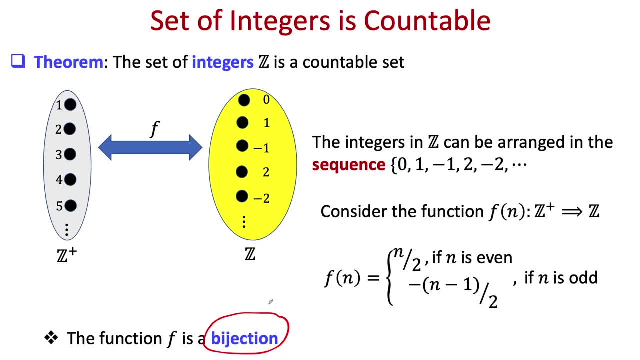 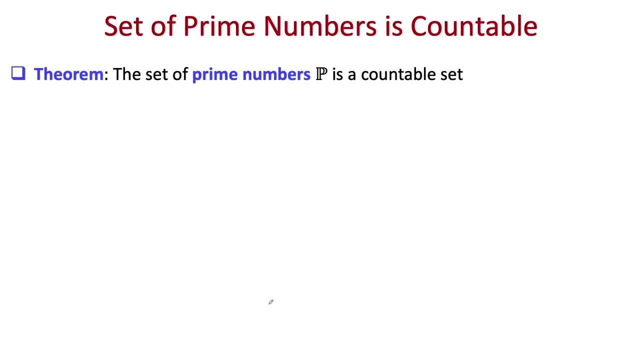 Which shows So? this shows that the cardinality of the set of positive integers and the cardinality of integers are the same. Next, let us consider the set of prime numbers. and for those who do not know what is a prime number, a number- P- is prime provided it is divisible by only 1 and P That means there. 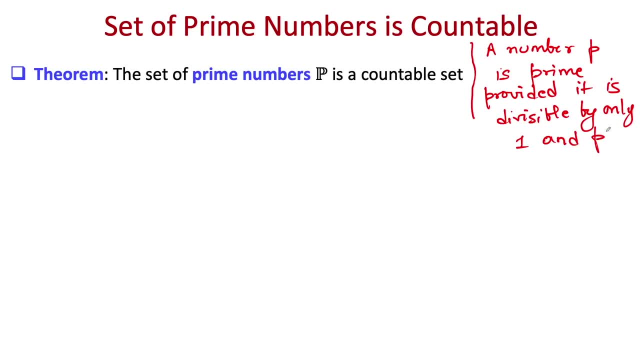 are no other divisors for the number P apart from the number 1 and the number P. Of course, 1 divides any number and the number divide itself By default. these are the two valid divisors of any number If your number P is such that you do not have any other divisors other than the number itself. 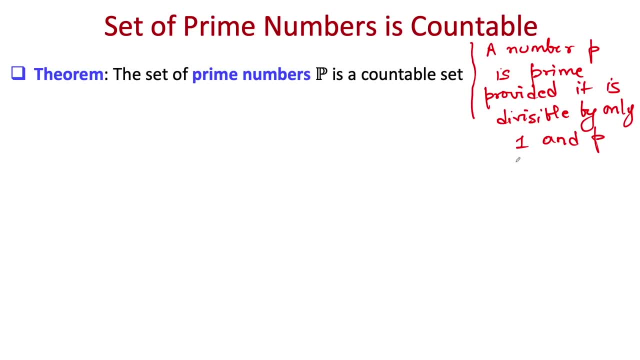 and 1, then the number P will be called as a prime number. So if you take, say, 2,, 3,, 5,, 7, they are all prime numbers, whereas if you take the numbers like 4,, 9, 15, they are not prime numbers. 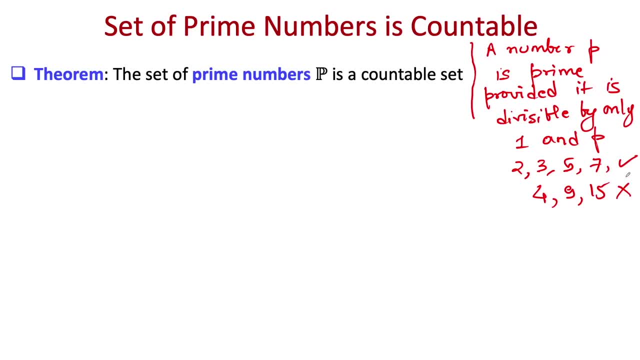 Because divisors of 4 are 2, divisors of 9 are 3, divisors of 15 are 3 and 5 and so on. So my claim is that a set of prime numbers is a countable set. So, again, those who are not familiar with number theory, they might be knowing that there are. 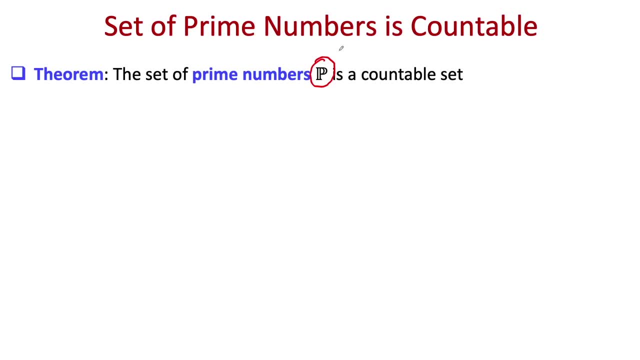 infinite number of prime numbers. But what we are stating in this theorem is that, cardinality wise, the number of prime numbers, The cardinality of the set of prime numbers, is same as the cardinality of the set of positive integers. So this I can either prove by giving you a valid sequence, and the sequence is very. 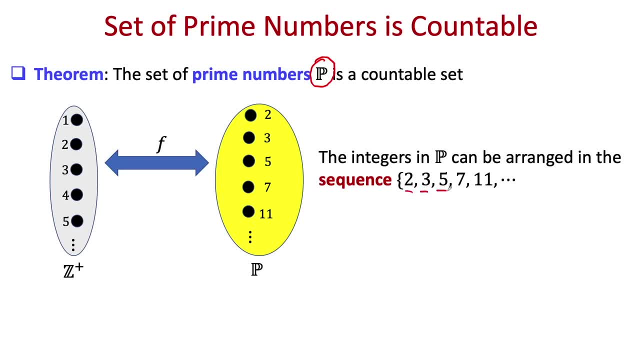 straightforward: You just enumerate the prime numbers in increasing order, that is all. and it is a valid sequence, because this is an infinite sequence. that is fine. So in the sense that every number in this sequence is a prime number, no number is going.